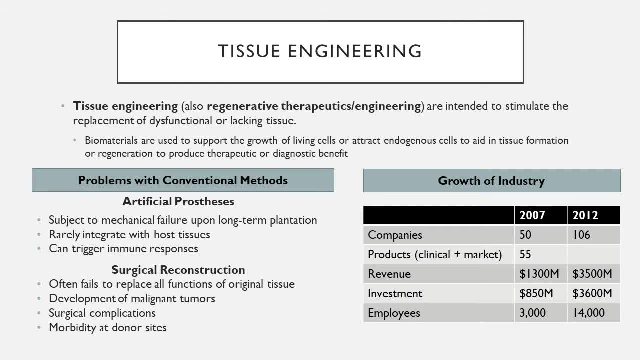 are used as a construct or a matrix to support the formation and growth of living cells and entrap them in the cell. So we've learned about the ability of cells to differentiate endogenous ones that aid in tissue formation and regeneration of the host tissue for some kind. 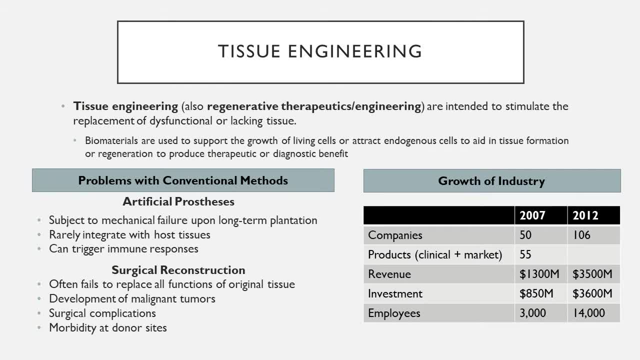 of benefit. right, And tissue engineering really came about probably in the early 90s as sort of a solution to conventional problems. with two separate approaches to solving these types of problems- okay, One would be. what we've been learning about the entire semester is the use. 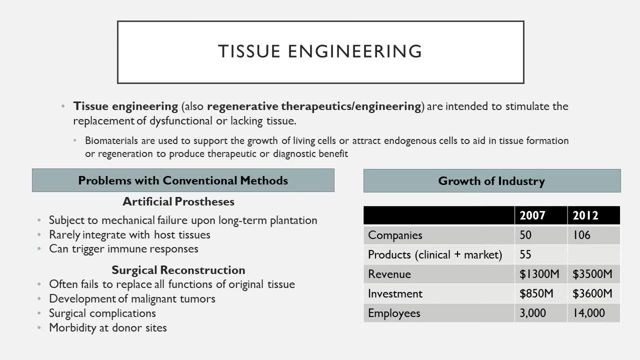 of artificial prostheses right. So we've learned that these are subject to a lot of mechanical failure upon long-term implantation. They rarely integrate themselves with host tissue in the same way that bones, tissues and joints typically do, And also here I'm lumping in the 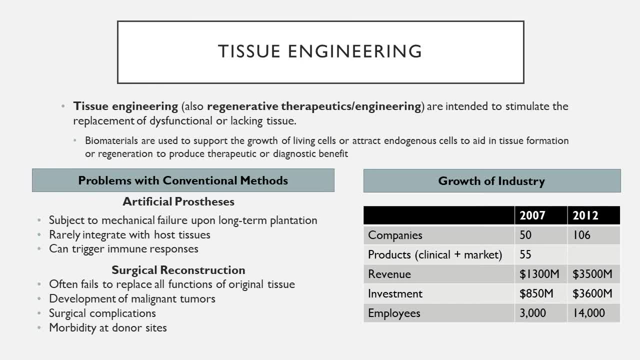 use of natural biomaterials that have either been donated, say from other sources, which themselves can trigger immune responses. okay. The other solution, perhaps a more conventional, non-engineering approach, is through surgical reconstruction. Okay. Now, in these cases, these often fail to replicate all the functional requirements of the 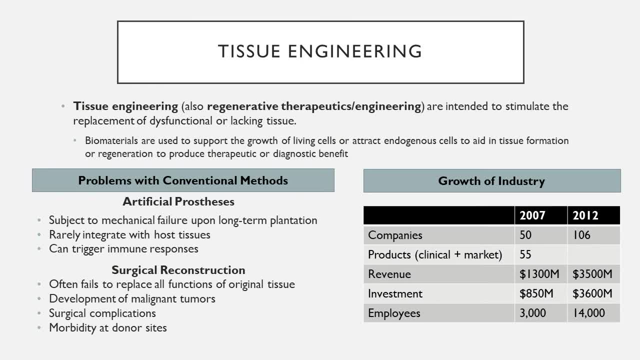 original tissue. They might be derived from other parts of the body. They have the potential for development of malignant tumors. Surgical complications arise where things just weren't restored to the natural function as they were intended. There's also morbidity at the donor site. okay, So the idea is that if you can just regenerate the healthy tissue to 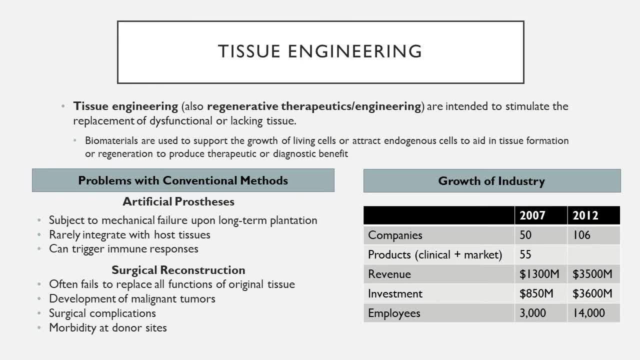 back to its original status or potentially even a more beneficial status, a higher than normal efficacy. then you can overcome all these conventional problems. Now the book kind of gives a few stats on the growth of this particular industry, particularly focusing on the 2007 years, And it gives a couple numbers. So 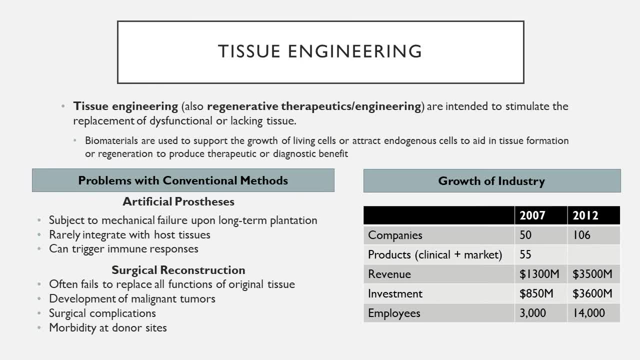 the number of companies that were around in 2007 numbered around 50,. all right, These companies have produced around 55 products that were either in the clinical stage or already on the market. Typical revenue was around 1.3 billion- The amount of investment. 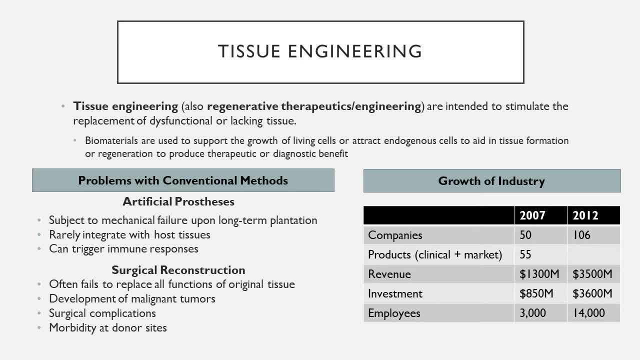 was close to a billion dollars. The amount of employees that were supporting this industry was around 3,000.. So here I've also attached a few numbers just five years from then, from 2012.. And these are some of the more up-to-date numbers that I could find. The number of companies has 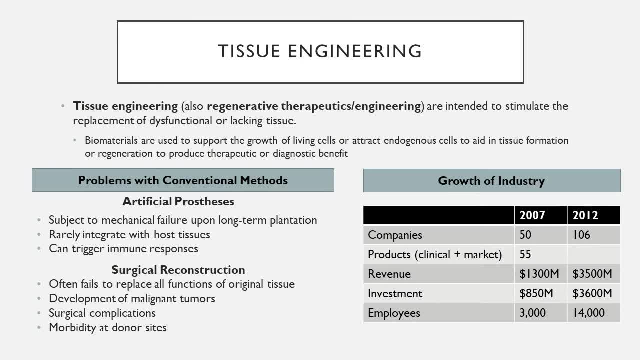 more than doubled. The amount of revenue has increased to about three and a half billion dollars. The amount invested same, about three and a half billion dollars as well. The number of employees has jumped almost an order of magnitude of 14,000, right, So an incredible jump just in that time span. Now, first, I'd like to give 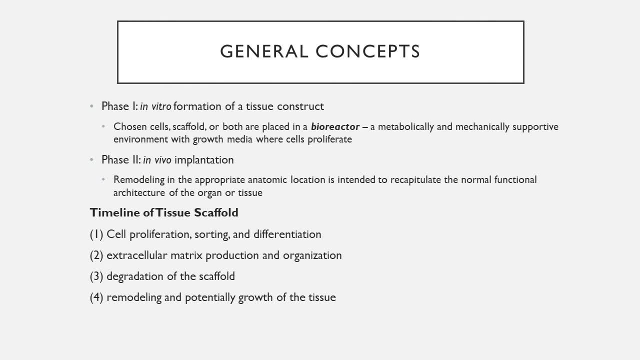 a general approach to a tissue engineering procedure. okay, This is just a generalized concept, but the first phase in tissue engineering typically requires the in vitro formation of a tissue construct. okay, Here cells, some sort of scaffold, are combined together and placed in what's called a bioreactor right. So this is a vessel that. 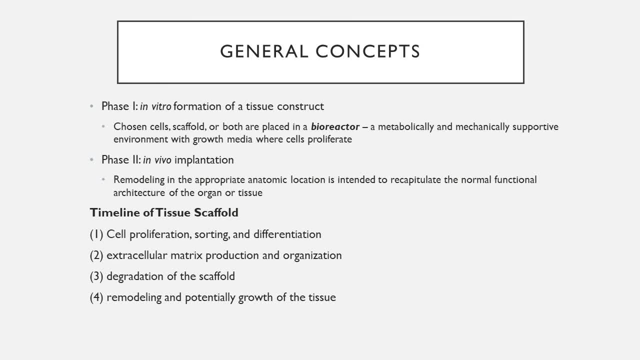 has the metabolically and mechanically supportive environment in which cells can grow- right With the growth media right, And here cells proliferate and elaborate. extracellular matrices that sort of provide the foundation of tissue- all right. In the second phase you have the in vivo implantation of this tissue construct, all right. 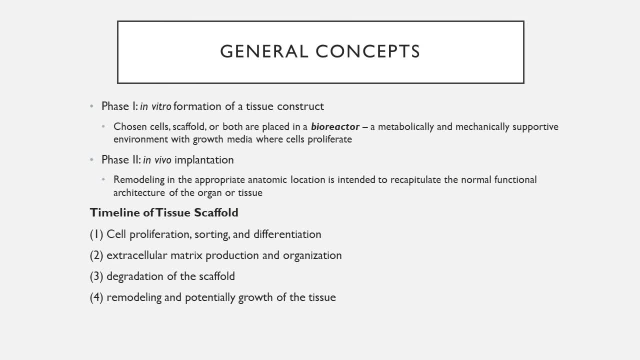 This is the remodeling of the in vivo is intended to recapitulate the normal functional architecture of an organ or tissue. all right, So the timeline of this typical scaffold is that first, cells proliferate, sort themselves and differentiate into the key cells required. 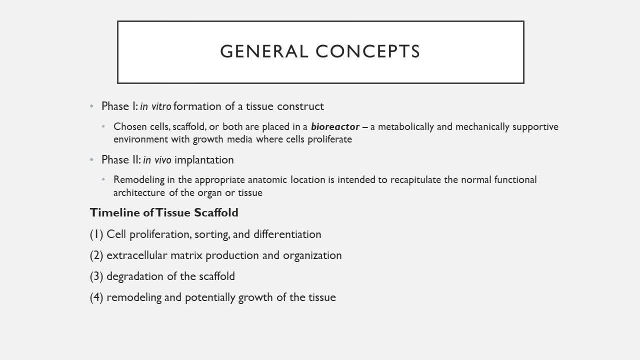 for that particular tissue. The cells then produce the extracellular matrix production and organize the sort of scaffold, the native tissue scaffold, as opposed to the one that was provided by the engineer. The third phase where we have our intended degradation of the scaffold that was originally produced. So this is what's going to the extracellular 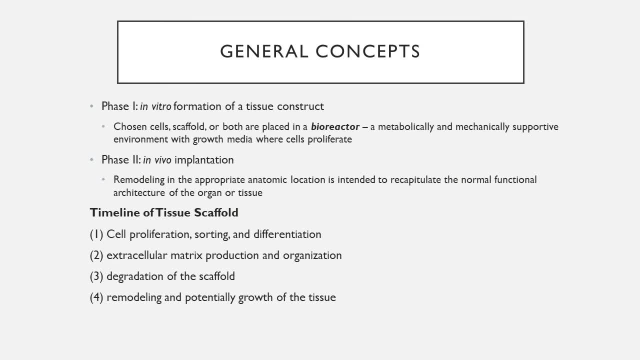 matrix is going to take the place of this, And then from there you have the remodeling and potential growth of tissue that arise from the combination of all the cells that are proliferating. This generalized strategy is shown here, pictured on the left, right. 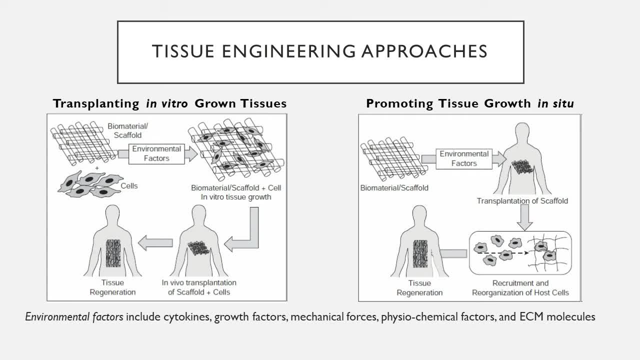 The in vitro grown tissues that are grown in a vitro stage and then implanted later in situ. This is in contrast to a secondary approach, which requires promoting tissue growth in situ. okay, Here the biomaterial scaffold is placed in vivo at the start and then cells are introduced. 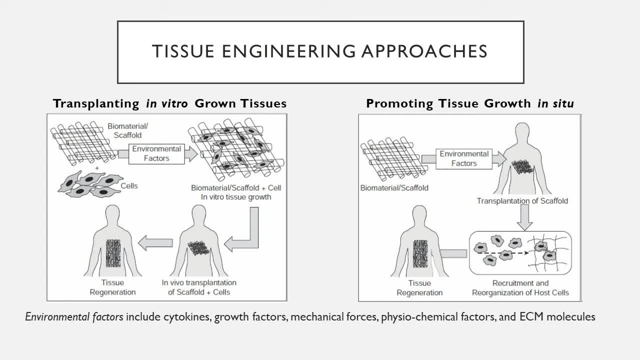 by the host — typically through the use of environmental factors like cytokines, growth factors, mechanical forces. Previously we talked about the inducement of M2 macrophages that help with the revascularization and angiogenesis of these scaffolds. 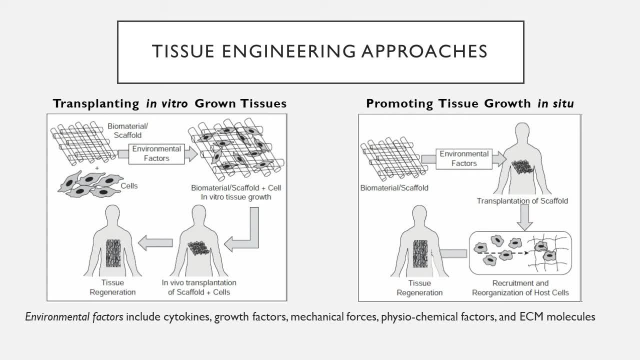 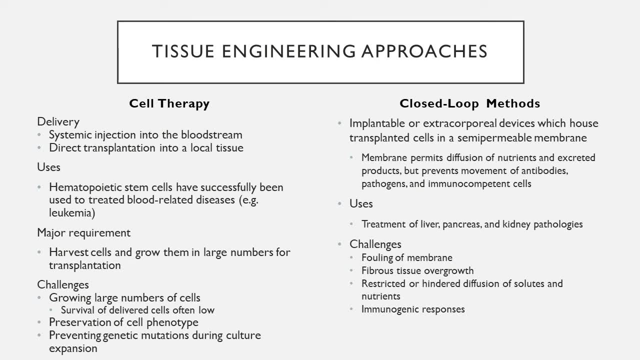 So these are two kind of generalized approaches to tissue engineering. Now, in addition to the two classical approaches of in vitro forming and in situ forming tissue engineering constructs, there's also two methods here called cell therapy and closed loop models that, while themselves not classically labeled tissue engineering approaches. 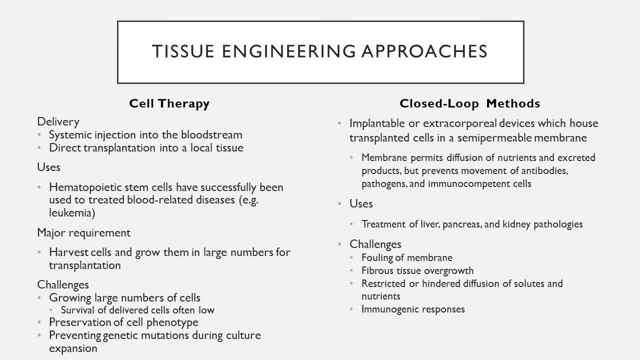 have themselves contributed greatly to our knowledge of our current understanding of tissue engineering. Cell therapy involves delivery of cells through systemic circulation into the bloodstream or through direct transplantation in the local tissue. The major requirement for this strategy is to harvest the cells and grow them in large numbers. 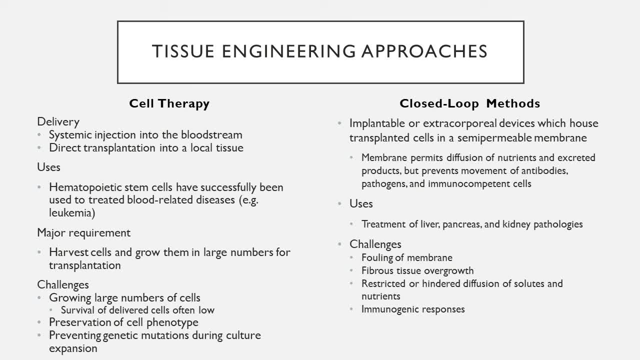 for in vivo transplantation. Now, direct injection of cells to the site is a common strategy to promote tissue regeneration. One of the major drawbacks is that the survival of delivered cells is typically low, often because the constructs lack a nutrient-rich environment and oxygen supply. 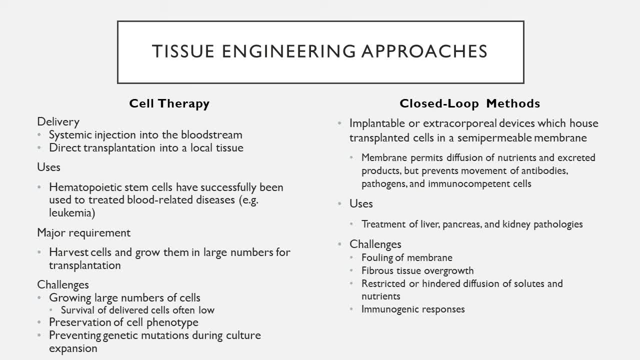 Now, alternatively, cells can be administered through systemic injection, which relies on the cell's tractors to produce the cells. So the cells are not able to travel through the circulation until they target the desired site or location. Now, because targeting specific sites, 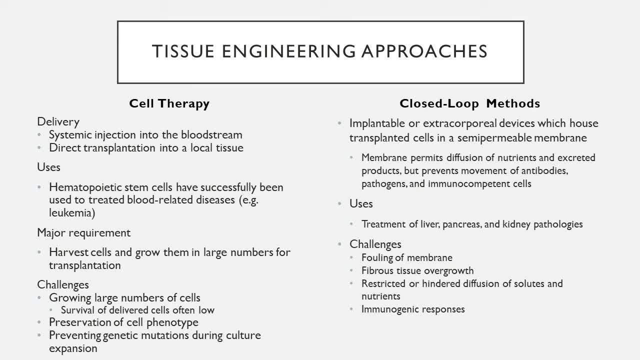 through nonspecific administration through systemic circulation is often difficult. we have seen a lot of early success in this method for the treatment of blood-related diseases, including leukemia, multiple myeloma and immune deficiencies. So you see this law with hematopoietic stem cells. 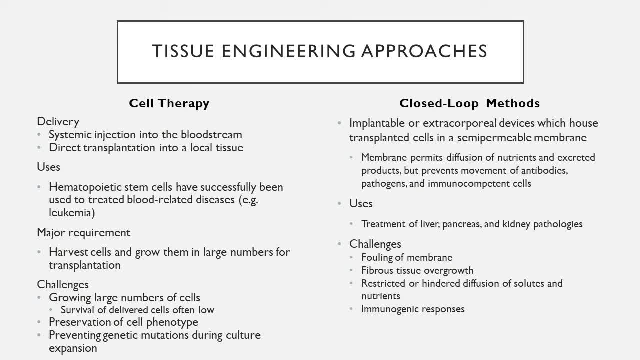 to treat blood-related diseases. So you see this law, with hematopoietic stem cells to treat blood-related diseases. Now, some of the main challenges for cell transportation are growing a large number of cells without bacterial contamination. This is in large part, required because of the low survival rate. 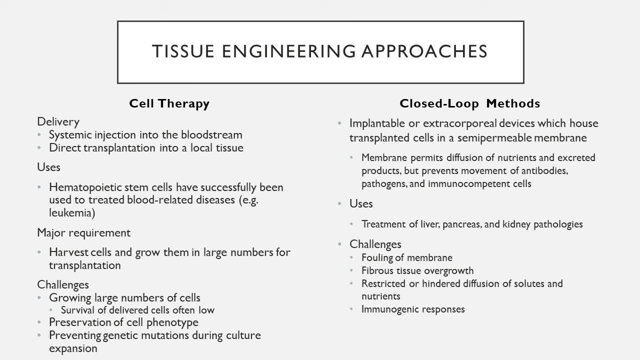 of cells that are administered. There's also the preservation of cell phenotype, So we learn about all the different ways in which cells can be induced to differentiate, and sometimes it's difficult to actually prevent that from happening, just due to the wide variety of environments that the cells are subject to. 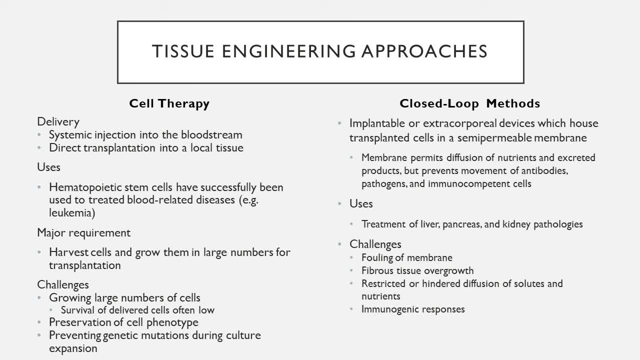 There's also preventing genetic mutations that occur during the culturing process and expansion. So all these challenges tend to result in the widespread death of the transplanted cells, poor engraftment and then also loss of control over the fate of the transplanted cells. 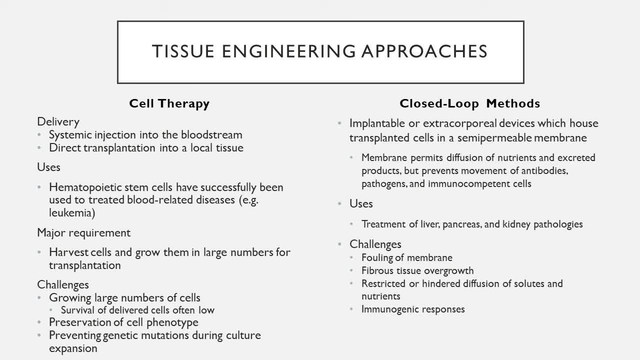 whether or not they differentiate in the type of phenotypes that are undesired for that type of cell, or they don't even go to the intended target site at all. An alternative strategy, called closed-loop methods, involves transplanted cells that are housed in a semipermeable membrane. 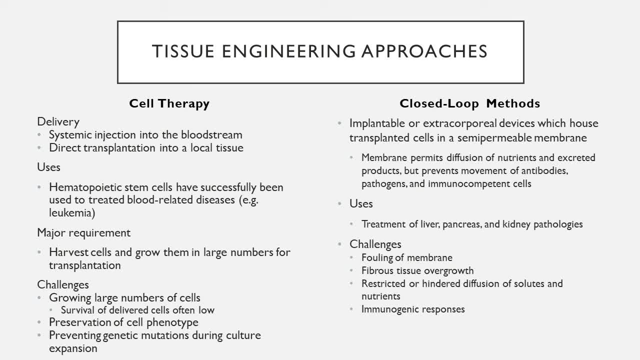 either outside the body, meaning extracorporeal, or actually implant in the body, yet separated from the rest of the tissue And the membrane, permits the diffusion of nutrients and excreted products, but prevents the movement of antibodies, pathogens and other immunocompetent cells. 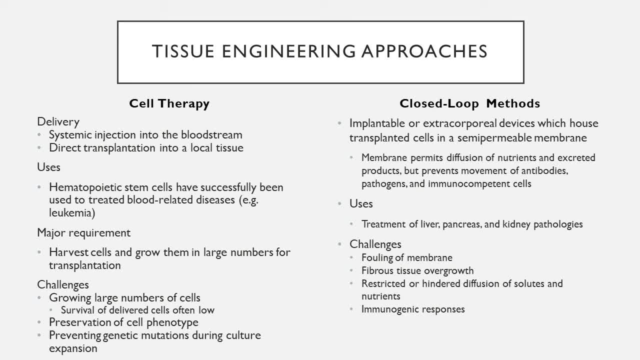 So oftentimes these don't even require host cells, tissues, just the function Of whatever donated tissue or cells that are required for that particular application. Now, when we think semipermeable membranes and the exchange of nutrients and products, of course this kind of makes us think of liver pancreases. 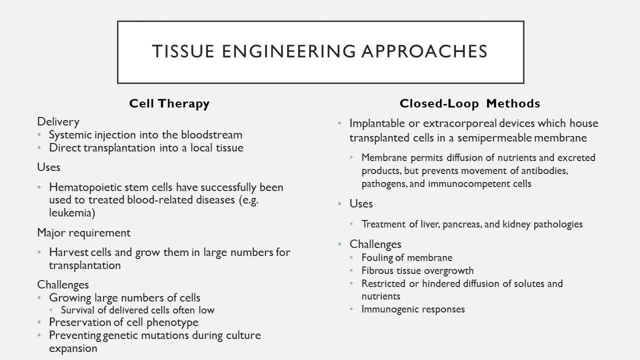 and kidney pathologies, which is where we see this type of closed-loop methods being implemented Now. major problems associated with these types of devices include fouling, fibrous tissue, overgrowth, restricted, hindered diffusion and also immunogenic responses, despite that sealed-off environment. 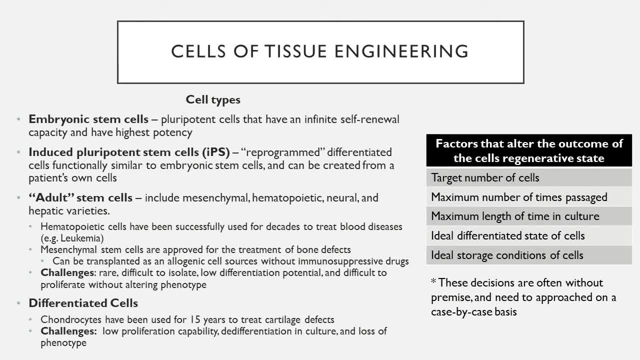 Now, there are a variety of components that go into tissue engineering. The first one that we're going to cover are the building blocks of tissues, which, of course, are cells. Now, cells involved in tissue engineering can either be stem cells that have the ability to differentiate into whatever cells. 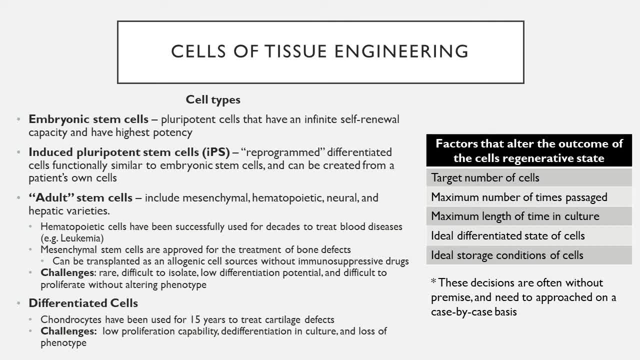 we'd like them to differentiate into, or also fully differentiated cells, meaning ones that have that have reached their full maturity and are already functioning in that specific state of whatever cell is desired. Now, many of these concepts we've covered previously in the background chapters in section two. 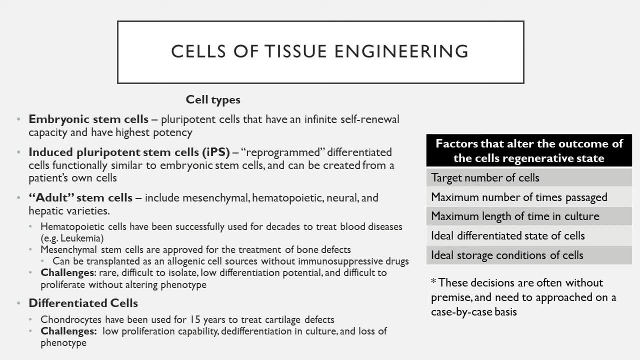 but embryonic stem cells are often thought of as the gold standard, because these are pluripotent stem cells that have an infinite capability of cell renewal and also have the capacity to differentiate- a term that we use here is potency- To differentiate into any of the 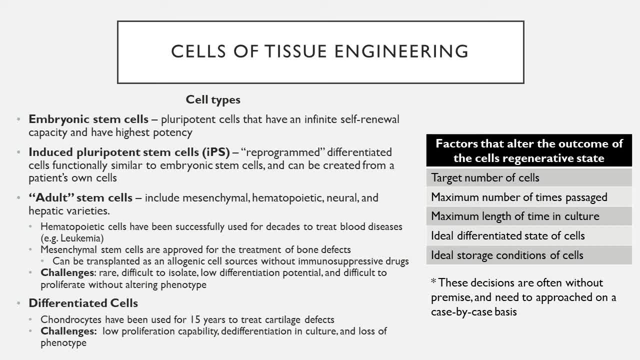 I think it's 213 types of cells found in the in humans. Now, adults also have their own types of stem cells, such as hematopoietic stem cells, which give rise to all types of leukocytes, mesenchymal stem cells, neural blood cells. 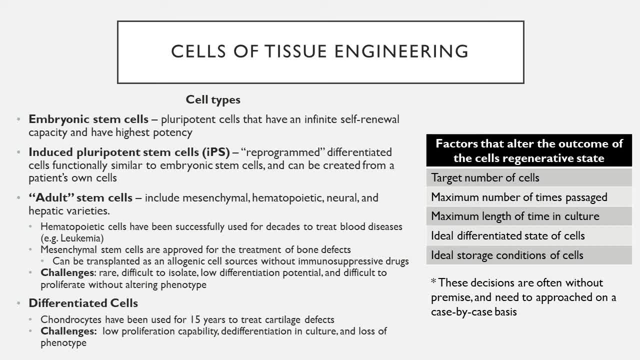 and a couple of hepatic varieties. As I mentioned in the previous slides, hematopoietic stem cells have been used for a few decades now in cell therapy for the treatment of various blood-borne diseases, Mesenchymal stem cells which give rise to various types of bone cartilage. 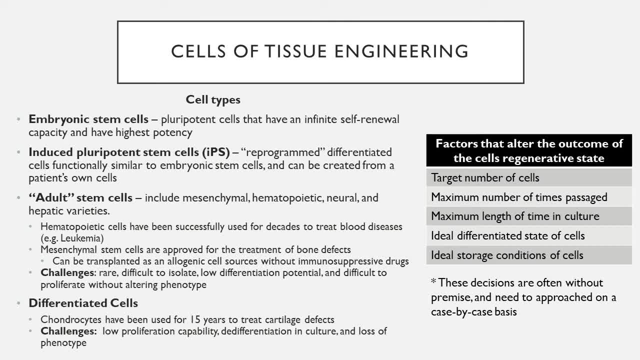 and muscle tissue have been approved for the use in multiple systems that treat bone defects. Nevertheless, adult stem cells are rare, challenging to isolate and expand without altering cell phenotype and limited in their differentiation potential. These type of adult stem cells are multipotent. 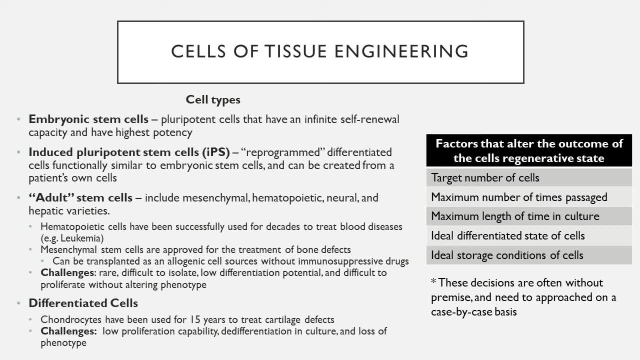 meaning they have a reduced capacity to differentiate and also proliferate in the form of self-renewal, in contrast to embryonic stem cells, which are pluripotent. Now an exciting new venture that has come about in recent decades is the idea of induced. 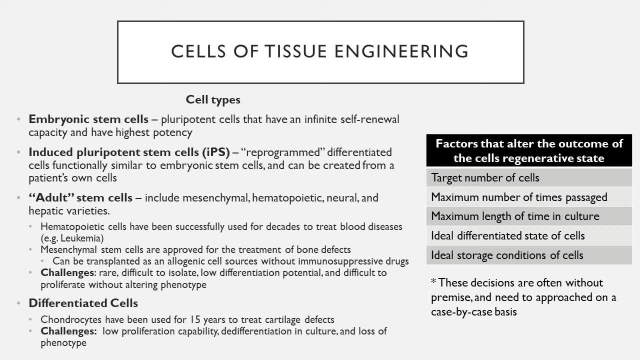 pluripotent stem cells, right? So these are reprogrammed differentiated cells that function very similar to embryonic stem cells and can be created from a patient's own cells. That last part is perhaps the most important part. Not only are they pluripotent, 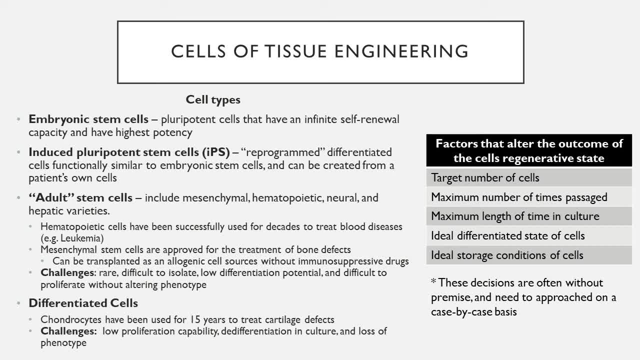 but they're also can be derived from host tissue, whereas it's typically very hard to harvest the adult stem cells mentioned previously. Now, when working with these types of cells, care must be taken during the cell isolation process in order to maintain cell phenotype purity and their differentiated state. 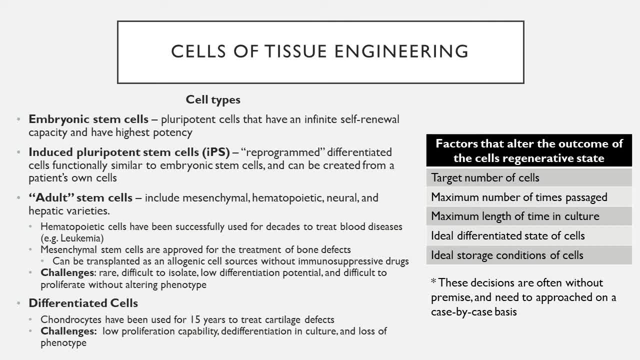 Okay, and there are a number of decisions that must be made, often without a suitable premise, such as the ideal number of cells to be transplanted or the ideal number of cells to be transplanted, the maximum number of times the cells can be passaged. 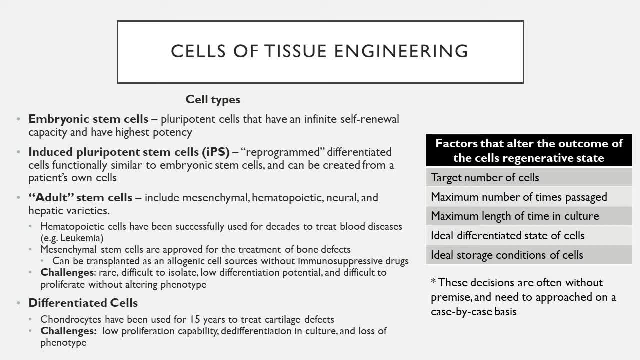 the maximum length of times the cells should be maintained and cultured, the ideal differentiated state of the cells to produce a therapeutic effect and, lastly, the ideal storage conditions of these cells, And oftentimes these have to be determined on a case-by-case basis. 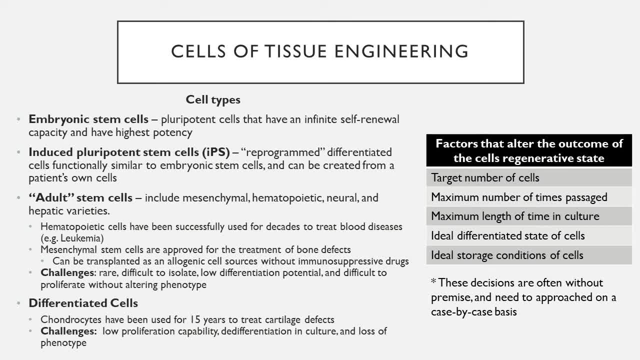 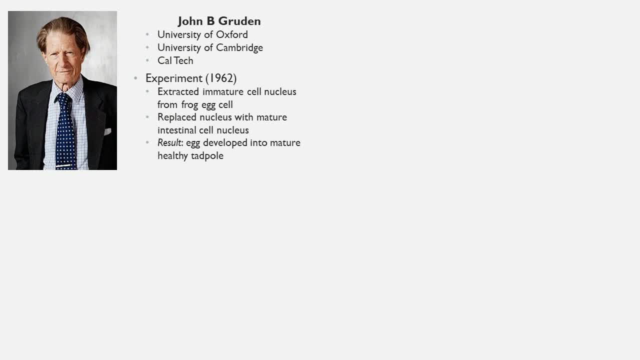 for specific people or animal models. Now I want to take a quick time out and tell a few very interesting and noteworthy stories revolving around this. I'm going to start off by talking a little bit about my friend John Gruden, who was a researcher at both Oxford University and also Cambridge. 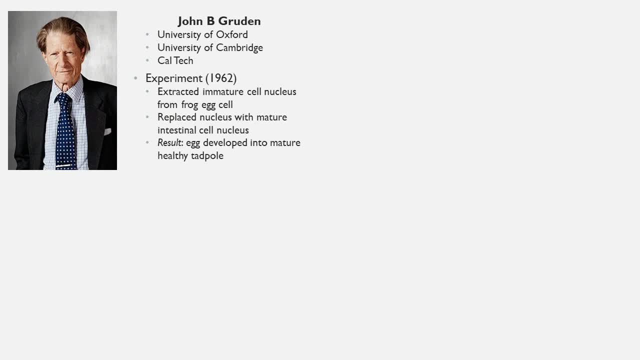 and later on Caltech. Now he had this landmark study in 1962 in which he extracted an immature cell nucleus from a frog egg cell, replaced that nucleus with a mature cell nucleus that was derived from a frog intestinal line and then he used that cell nucleus to extract a new cell nucleus. 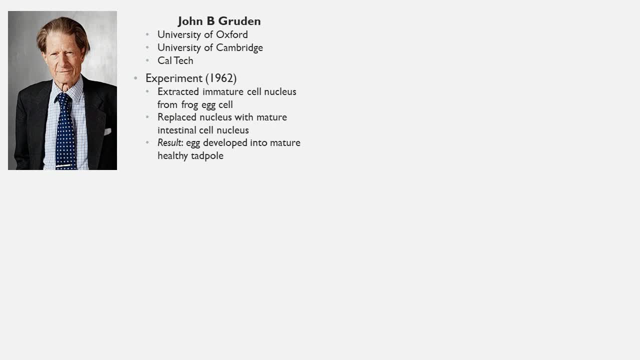 from a frog egg cell. Now, this cell nucleus was derived from a frog intestinal line, and the result of which is that the egg, despite having this mature nucleus, still developed into a normal, mature, healthy tadpole, And the conclusion that was taken away from this is that 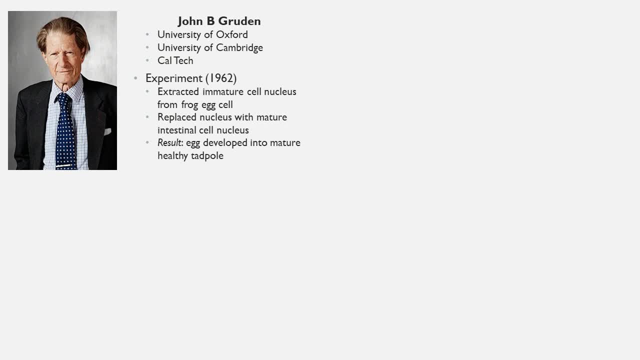 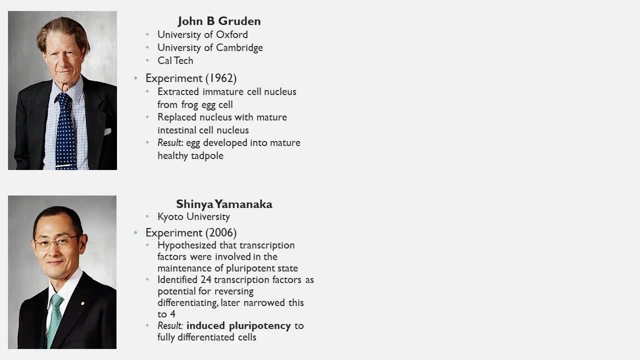 there are factors that can induce that sort of pre-differentiated state from a fully mature cell. And this all happened in 1962, but in a much later study, and more recently in 2006,, Shinya Yamanaka from Kyoto University in Japan. 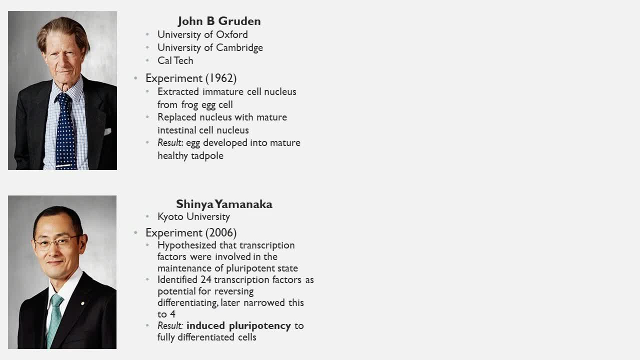 hypothesized that there are genetic and transcription factors involved in maintaining the pluripotent state of these immature cells. So he at first identified 24 transcription factors that later he narrowed down to four and isolated these transcription factors and then introduced them into fully differentiated cells. 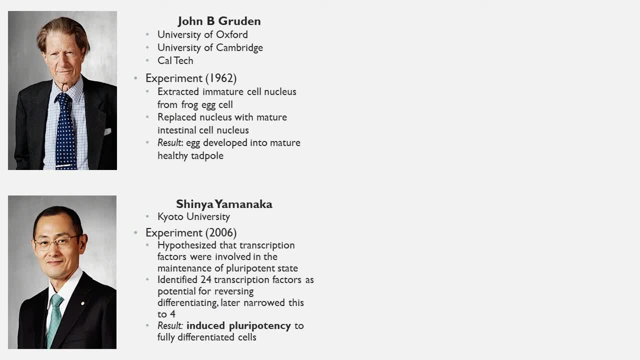 And what he got was the inducement of a renewed and sort of embryonic state of these stem cells from fully differentiated cells, And this was sort of a landmark case, and the basis of these two works resulted in the 2012 awarding. 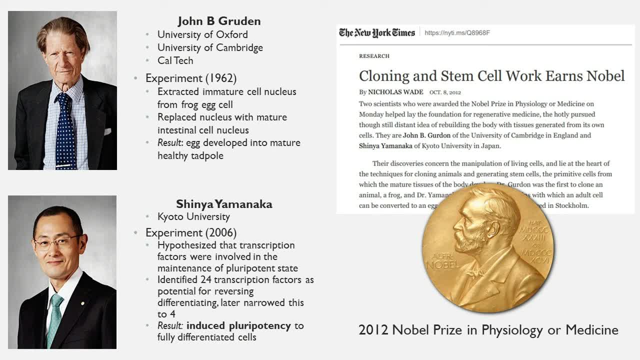 of the Nobel Prize in Physiology or Medicine to both of these researchers. So one kind of came up with the idea of inducing a pluripotent state and then later on figure out a mechanism for which to induce that Now, working with gene and transcription factors. 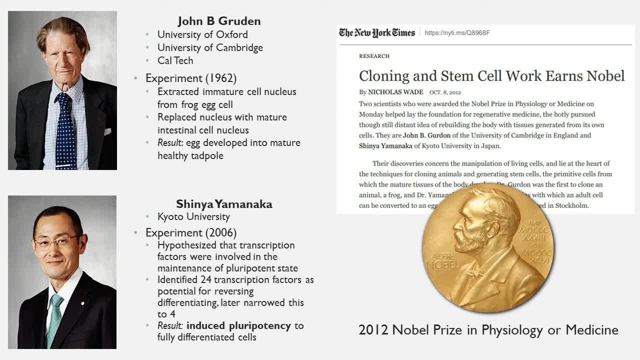 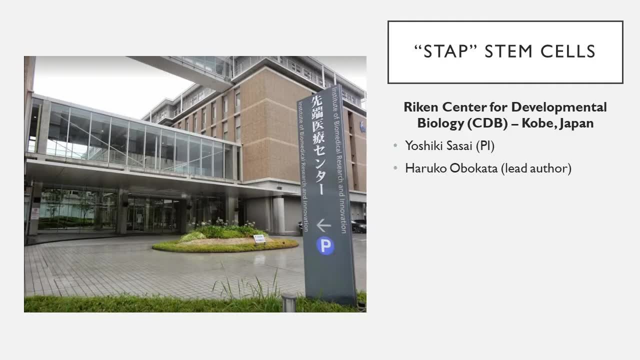 in order to alter cells and induce the pluripotent state, as you can imagine, is rather difficult and not everyone is capable of doing it, So there is a lot of excitement around. this was 2013,, 2014,- when two articles from Nature came out. 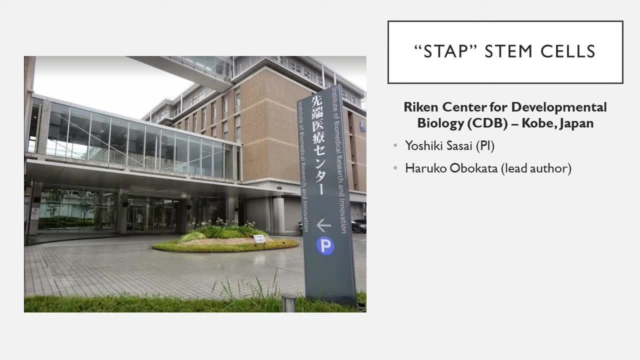 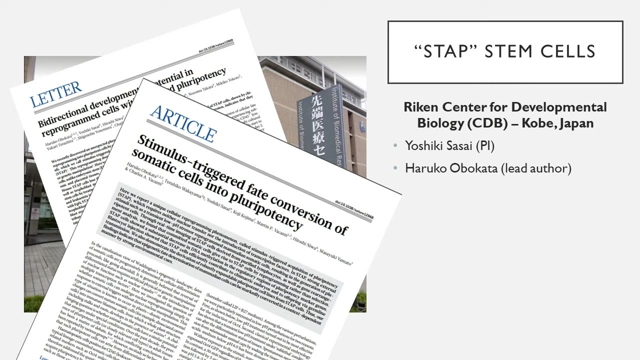 that originated from the Reichen Center for Developmental Biology in Kobe, Japan, In particular two researchers: the PI of this research facility, Yoshiki Sasai, and his main researcher and the first author on both of these papers, Haruko Obakata. 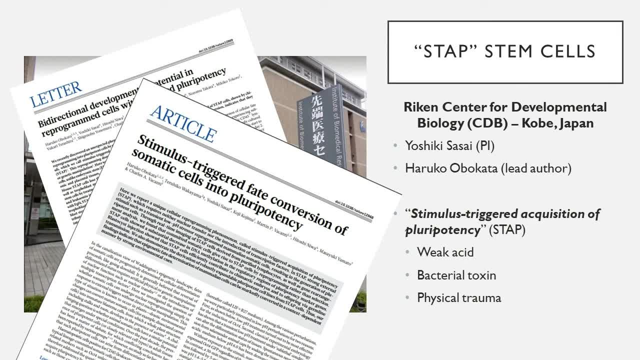 developed a way to induce this pluripotent state simply through external stimuli. So they had the idea that if you can induce this sort of harsh environment, and they had a couple different ways of doing this, whether through acidic baths, bacterial toxin or even physical trauma- 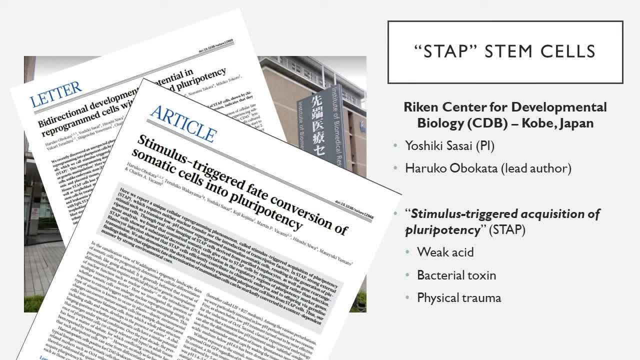 they could reverse the differentiated state of fully mature and differentiated cells back to their pluripotent embryonic state, And I can't stress enough how groundbreaking these works were, In contrast to the previous study where a researcher in 2006, using pretty complex methods, 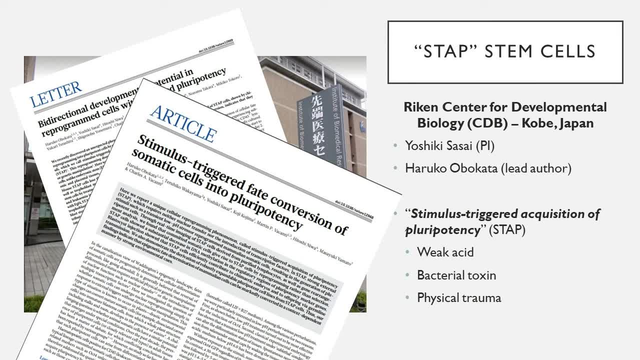 to alter the genetic state, thus reversing the differentiation of these cells, resulted in a Nobel Prize just six years later. work like this that claimed to have such much more simpler methods that anyone had access to, was guaranteed to not only get prizes like the Nobel Prize. 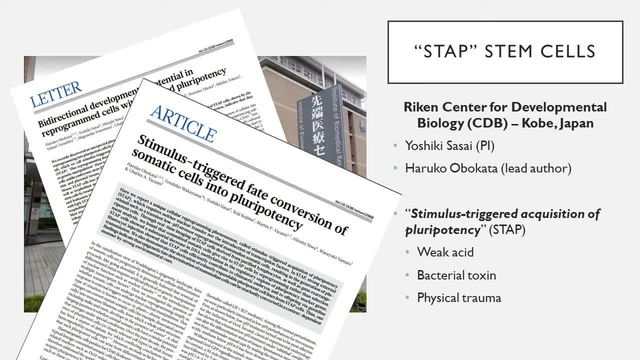 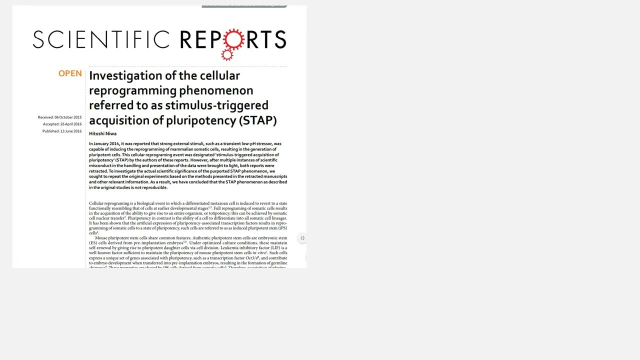 but also just alter entirely the way we go about doing research. It can't be stressed enough. So, of course, every lab around the world had a strong interest in pursuing this type of work. Now, unfortunately, attempts to recreate these results resulted in failure by 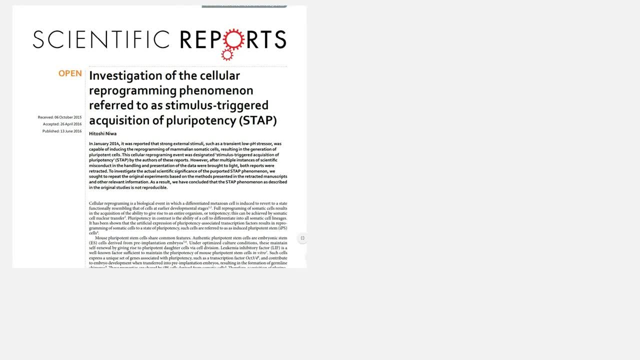 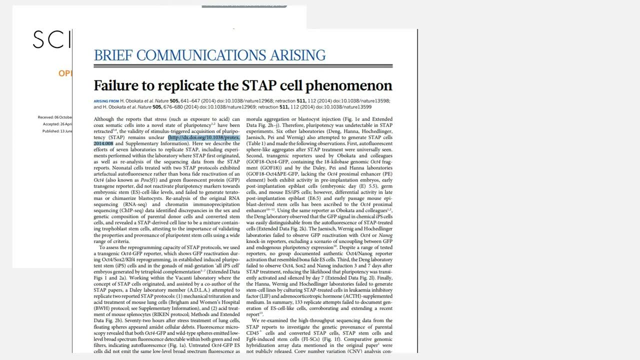 anyone else who tried to replicate them. Most of the time, cells ended up dying due to the distressed nature. No embryonic stem cells were induced And there are even a large amount of publications that discuss the failure of replicating these original results. 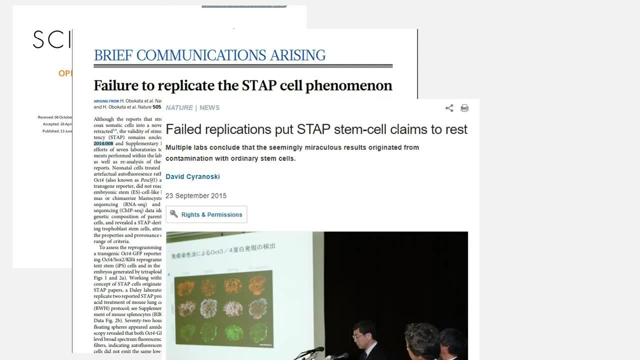 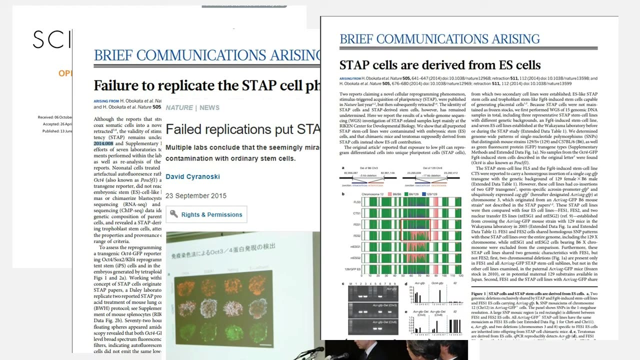 And eventually evidence mounted so much of these failed replications that it was eventually decided that this was not a viable study. These were not viable methods, despite what was published previously, And in fact later on it was found out that embryonic stem cells were. 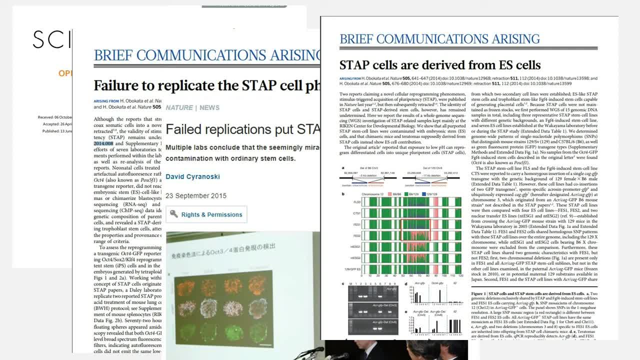 quote-unquote- contaminating the original results, And this is really sort of a nice way of saying that the authors likely implanted the embryonic stem cells separately from the results that they were trying to get, In fact, faking their results. Now, as you can imagine, 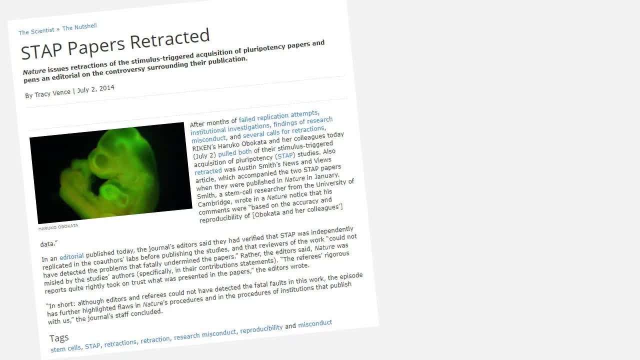 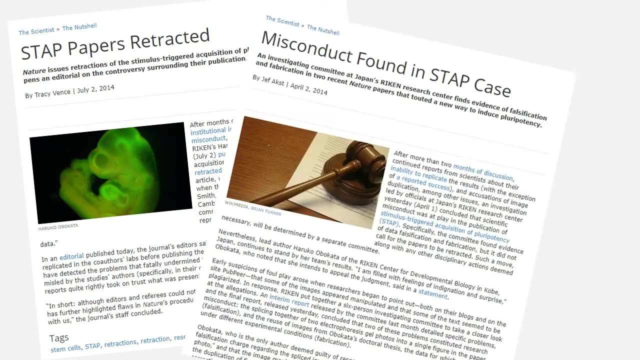 there are a lot of consequences that resulted in this. Of course, the two Nature publications articles were retracted, A highly embarrassing move, not only for the journal- this highly reputable and respected journal- but also, of course, the researchers. They had to admit they were wrong. 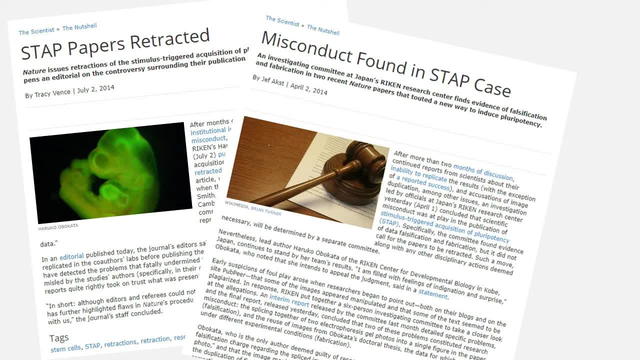 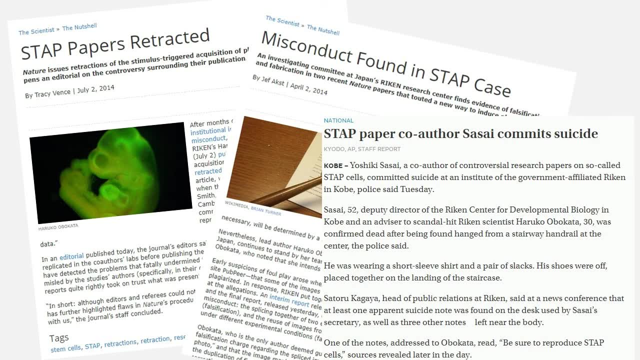 In fact there were investigations by the university, by the research institution itself, that found misconduct on the behalf of both researchers And, in a really unfortunate ending to the story, the lead PI of this research institute ended up taking his own life due to the scrutiny that this brought. 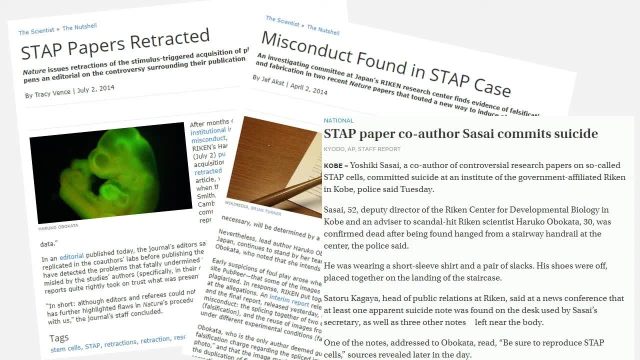 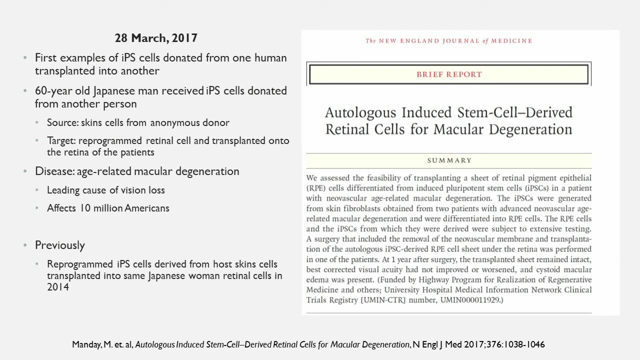 both the institution himself and his family. This story really represents one of the largest scandals in the research field, certainly in the past few decades and likely for some decades to come. Now, on the more exciting news front, just about a year ago today, 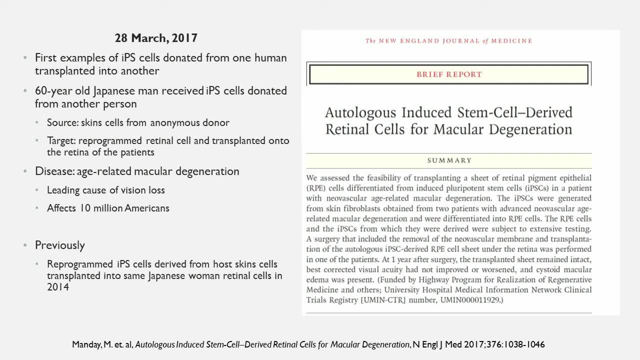 one of the first examples of induced pluripotent stem cells. these are through genetic transcription mechanisms, from one donor, human was transplanted into another human. In this case it was a 60-year-old Japanese man who received IPS cells donated from another person. 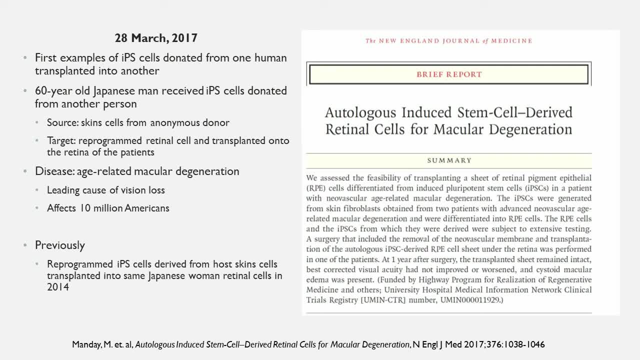 And the target was reprogrammed- retinal cells that were transplanted into the retina of this Japanese man, And the purpose of this was to treat this age-related macular degeneration of the eyes, one of the leading causes of vision losses that affects 10 million Americans. 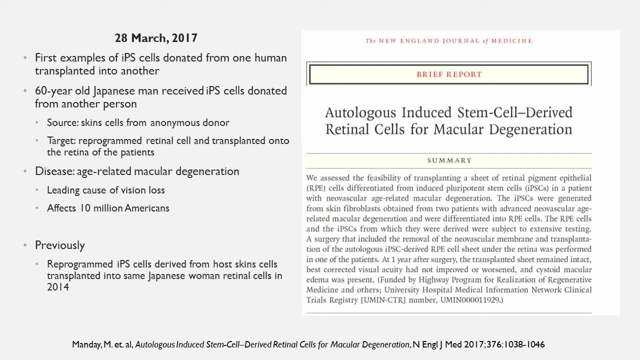 Now, before this, in 2014,, researchers had taken skin cells from one donor, reprogrammed them and implanted them into the same donor- in this case, this was a Japanese woman- for the treatment of the same disease. But just a year ago today, 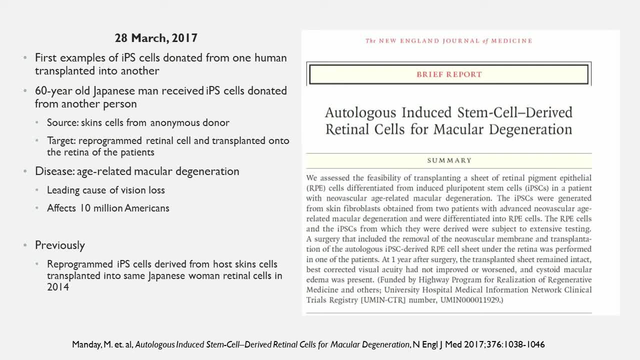 this was an example of using stem cells derived from a different donor and putting them into a separate recipient. So the idea that you can imagine, or sort of, in the future we would have banks of reprogrammed stem cells that could be implanted into anyone else. 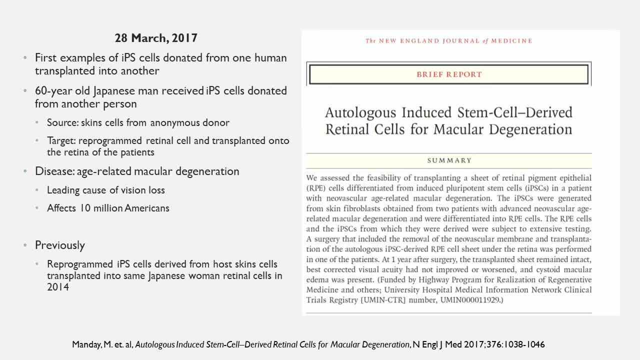 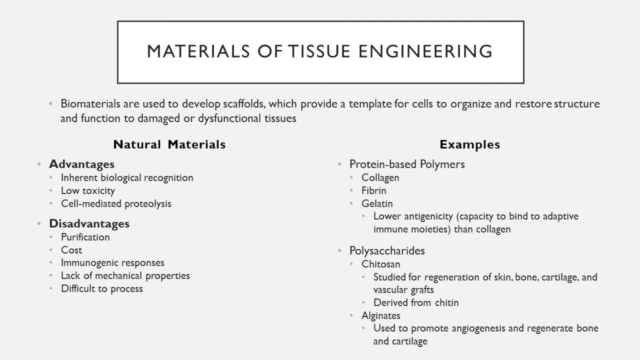 ideally with minimal immunogenic responses, and then use those cells for whatever disease treatment that we wanted. So this is really kind of research happening now. it's really exciting Now that we've discussed the main building blocks of tissues, that is, cells. 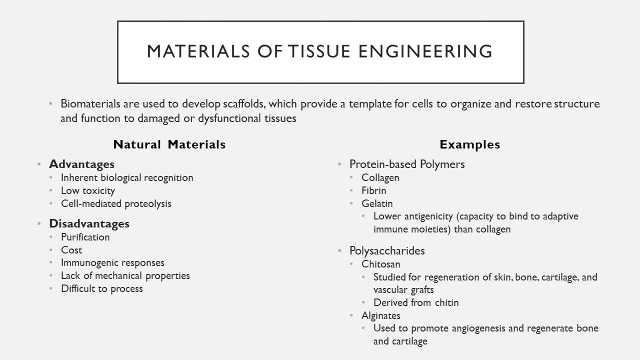 we come back to sort of the subject of this entire course, which are the biomaterials that are used in tissue engineering. In this case, biomaterials are used to develop scaffolds, which themselves provide a template or matrix for cells to organize and restore their structure. 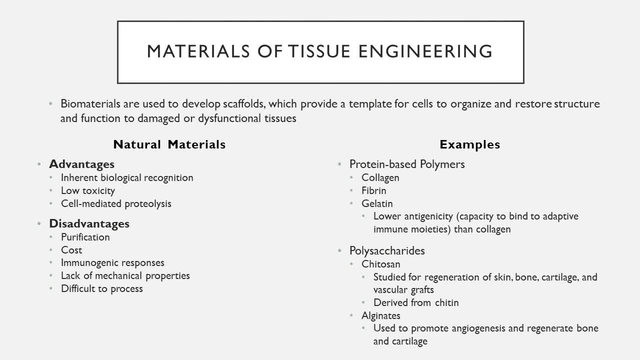 and functional damage or dysfunctional tissues. Now these materials can be divided up into two separate categories, One of those being made up of natural materials, which have several advantages. So one is having their inherent biological recognition through receptor-ligand interactions. cell-mediated proteolysis. 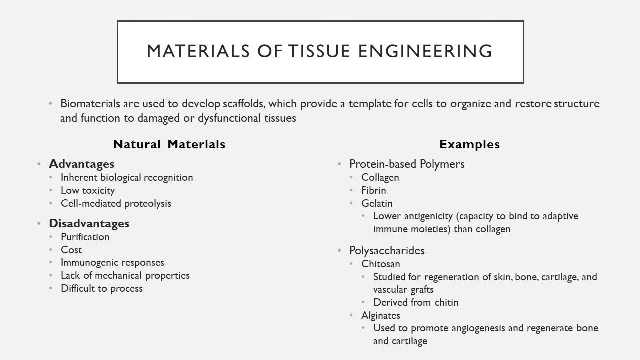 and remodeling, and also low toxicity. Classic examples of these would be protein-based natural materials such as collagen, gelatin, fibrin and elastin- Silk as well. Gelatin is a natural polymer derived from collagen, and what advantage it has over. 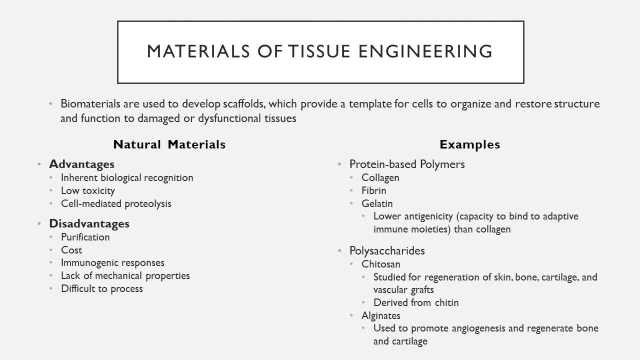 gelatin is that it has significantly lower antigenicity, which is the tendency to react with adaptive immune responses, such as through T-cells. Silk has also received a lot of attention due to this high strength to weight ratio and slow degradation. Polysaccharide natural materials include 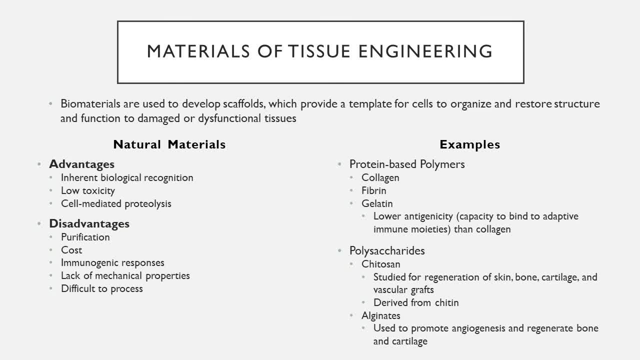 chitosan, which is self-derived from chitin and is studied for the regeneration of skin, bone, vascular grafts and cartilage, and also alginates, which are used to promote angiogenesis and regenerate bone and cartilage. Now, unfortunately, there are several limitations. 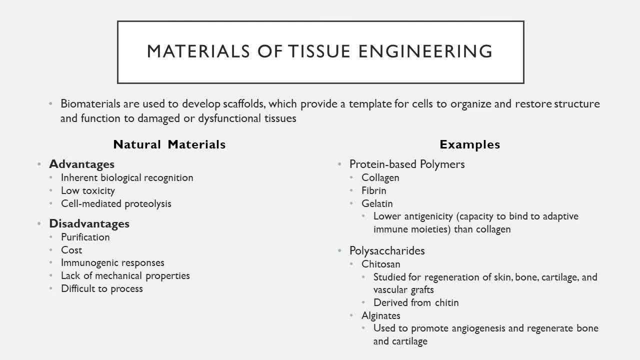 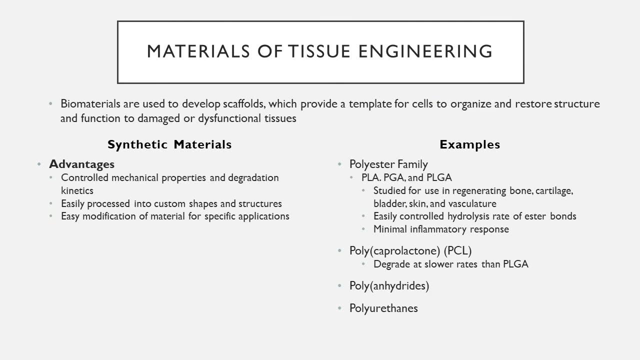 to natural materials, which include their purification cost, their potential for immunogenic responses and also the lack of mechanical properties and processability. Now, synthetic materials, on the other hand, have a lot of advantages that are in direct contrast to the disadvantages of natural. 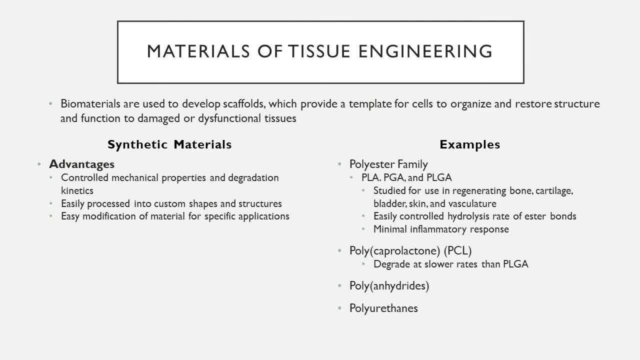 materials, such as the ability to control mechanical properties and degradation kinetics, their easy processability and accustomed shapes and structures, and easy modification of the material for various and specific applications. Some of the more common polymers that we see for tissue engineering applications would be polylactic acid. 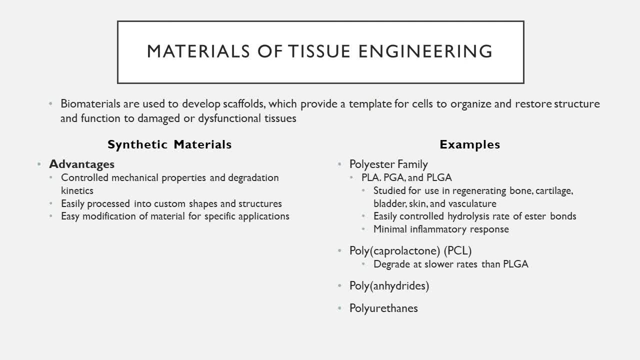 polyglycolic acid and the copolymer PLGA, combination of those two. We see it studied for a lot of uses in regenerative bone cartilage, bladder, skin and vasculature systems. They have really easily controlled. 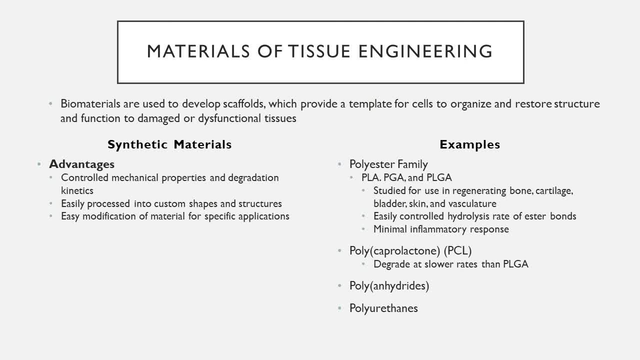 hydrolysis rates that can be tuned depending on the ratio of the glycolic acid and lactic acid. Remember that glycolic acid hydrolyzes faster than lactic acid and thus has faster degradation rates. Another very commonly used one is polycaprolactone, abbreviated PCL. 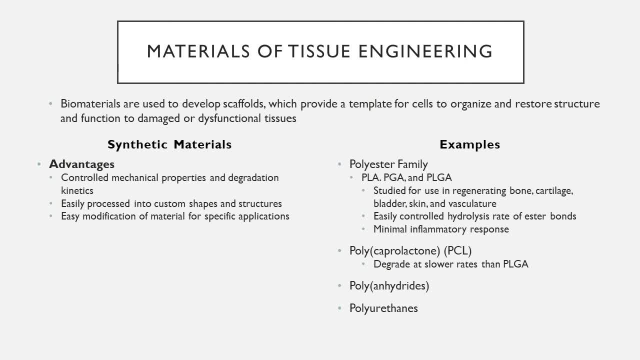 It tends to degrade at slower rates than PLGA. Polyanhydrides are one of the more faster degrading polymers. Remember that's a surface degradation phenomenon as opposed to the bulk degradation of PCL and PLGA, And also polyurethanes. 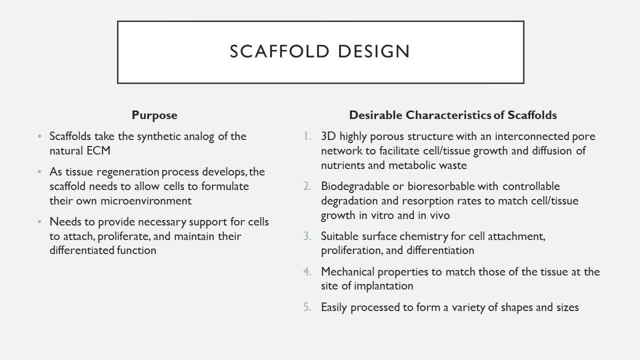 Once a proper material has been chosen, we want to incorporate that material into the design of a scaffold, The purpose of which is to recapitulate the normal tissue development process by allowing cells to formulate their own micro environment. In this case, the scaffold is really taking the place. 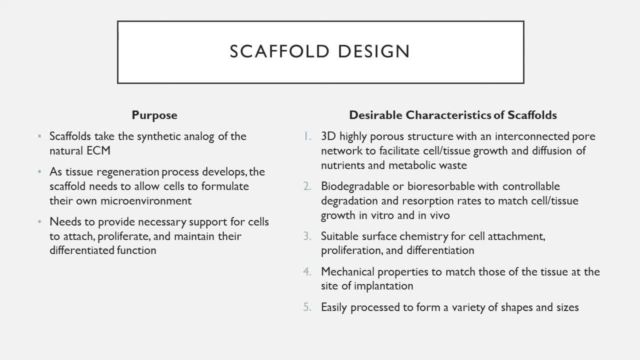 and is the synthetic analog of the natural extracellular matrix that cells produce and build around them. It needs to provide the necessary support for cells to attach, migrate, proliferate and maintain their differentiated function. In order to do so, these scaffolds need to. 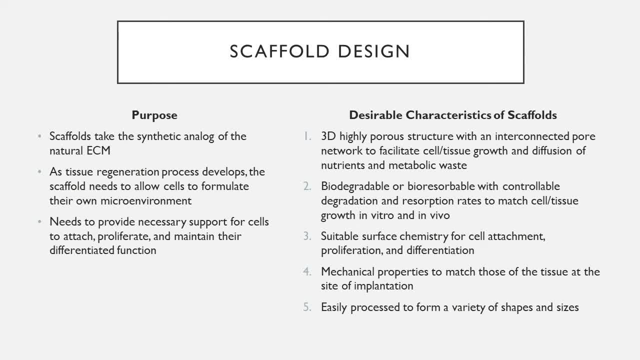 have five characteristic traits of them. The first is which to be a three-dimensional and highly porous structure with an interconnected pore network to facilitate cell and tissue growth and diffusion of nutrients, metabolic waste and paracrine factors. The second trait is that it needs to 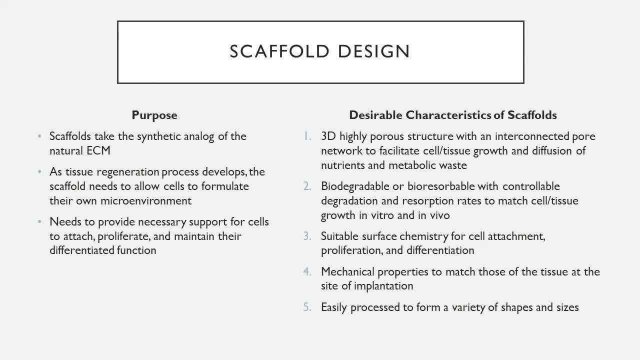 be biodegradable or bioresorbable, with controlled degradation and resorption rates such as to match the tissue or cell growth in vitro and in vivo, meaning that as the scaffold degrades, the tissues are being rebuilt and natural ECM is being built at that same exact. 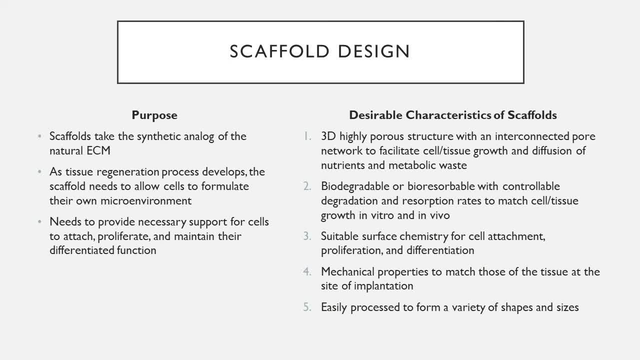 degradation rate in order to match and take up its place. The third characteristic is that it needs to have suitable surface chemistry for cell attachment, proliferation and differentiation. So remember, the attachment and migration patterns of these cells are highly dependent on their differentiation and vice. 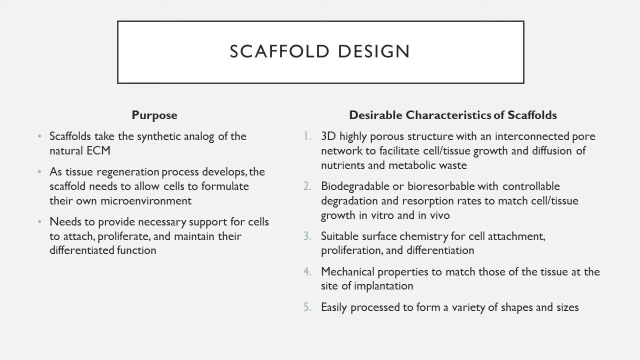 versa, Those cells, depending on what they attach to, are going to differentiate into different cells. These are stem cells we're talking about. The fourth characteristic is that it needs to have the mechanical properties to match those of the tissues at the site of implantation. So if it's 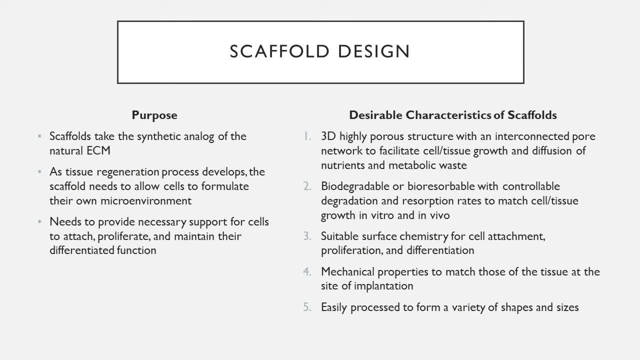 a soft tissue, a hard tissue, a ligament, collagen, soft muscle. it needs to have those same exact mechanical characteristics. And then the fifth characteristic is that it needs to be easily processed to form a variety of shapes and sizes to match its 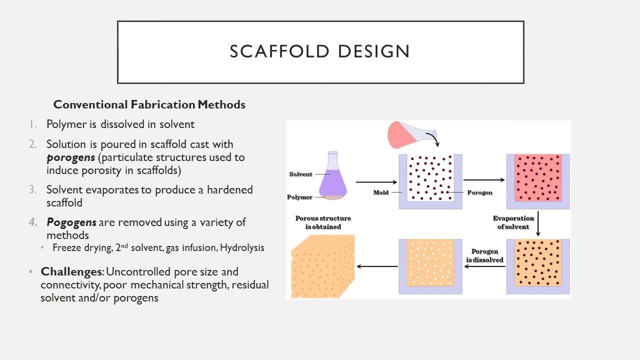 suitable design criteria. So now I'll cover a traditional method for developing scaffold designs: The first step, which involves dissolving polymer in a suitable solvent, typically one that's volatile and is going to evaporate easily. You then pour the solution into a scaffold cast. 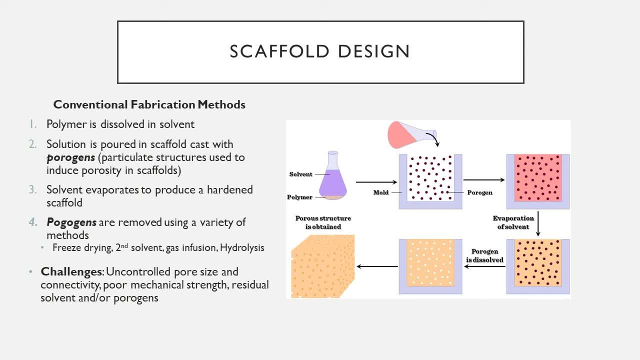 in combination with porogens, which are particular structures that are used to induce porosity in a scaffold, So they really just take up space, which will eventually form pores within the scaffold. You then allow that solvent to evaporate, leaving behind the precipitated polymer. 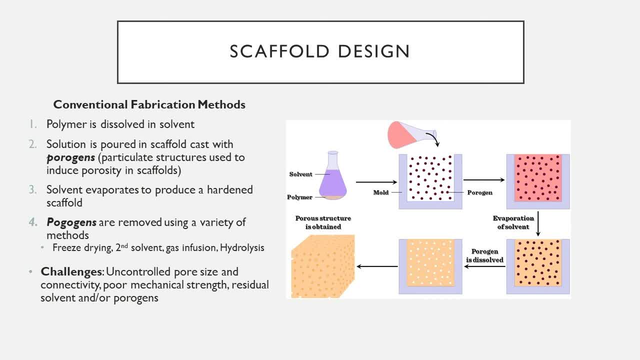 scaffold, Then those porogens are removed using a variety of different methods. This could be freeze-drying, using a second solvent that dissolves the porogen but not the scaffold gas infusion, or actually introducing degradable porogens that can hydrolyze and 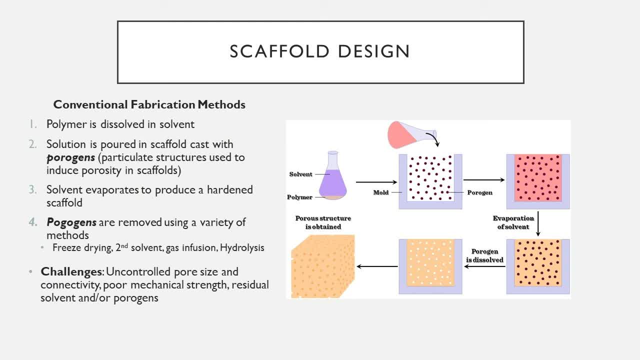 thus degrade, leaving behind that pore structure. Now, a couple of challenges with this particular design and fabrication method are the inability to control the pore size and connectivity of those pores. So not just making holes within the scaffold but making sure that those pores are interconnected. 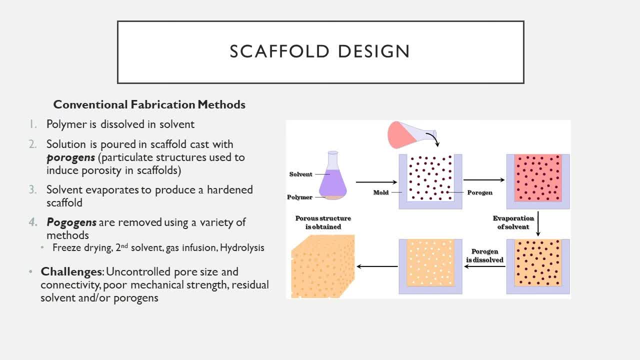 with each other. Poor mechanical strength, particularly with hydrogels. and then also residual solvent. Remember, if it's a volatile solvent capable of dissolving that polymer, it's probably not a substance you want in your body. And the same goes for 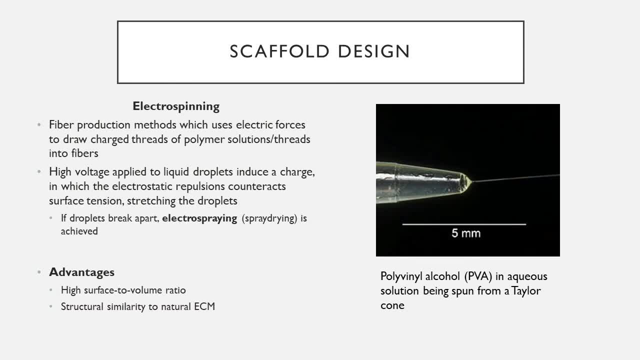 those porogens as well. Now a common technique for introducing fibrous scaffold designs is using the technique of electrospinning. Now electrospinning is a versatile process with high production capabilities and it's been used for a number of different designs. Dr Beachley uses this extensively. 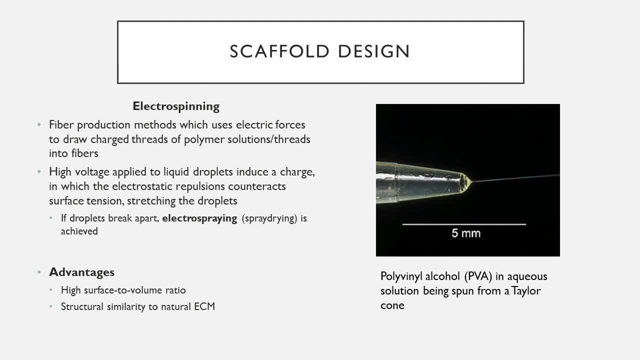 and if you've ever walked through the labs, you've likely seen someone electrospinning there. PCL is a very common polymer used for this. I've also seen POA applications or POA polymers used in these applications. Now, electrospinning involves using 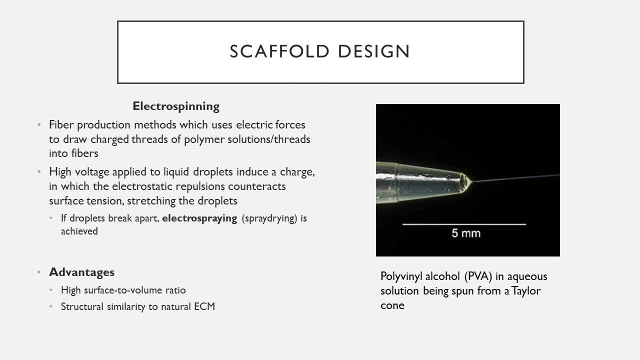 fiber production methods in which electric forces are used to draw charged threads of polymer in solutions into fibers. In this case, a high voltage is applied to liquid droplets to induce a charge and, when the charge of those forces are enough to overcome the surface tension, a thin polymer jet. 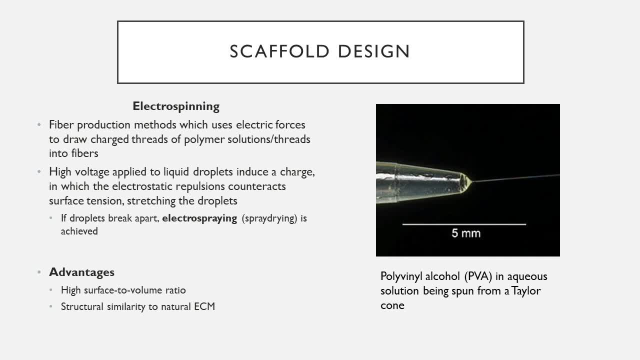 forms. Now, as these liquid jet streams are formed, the solvent that's dissolved, the polymer, would evaporate, leave behind these woven fibers. Now, in the cases where the droplets break apart, then you have what's known as electrospraying, or 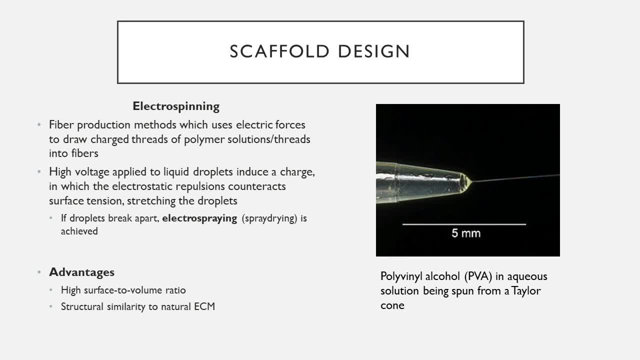 spray drying, which is very often utilized in the production of nanoparticulate drug delivery, due to the very small droplets that can be formed using this technique. So some of the advantages of this technique are the high surface to volume ratio of the fibers and also the structural similarities. 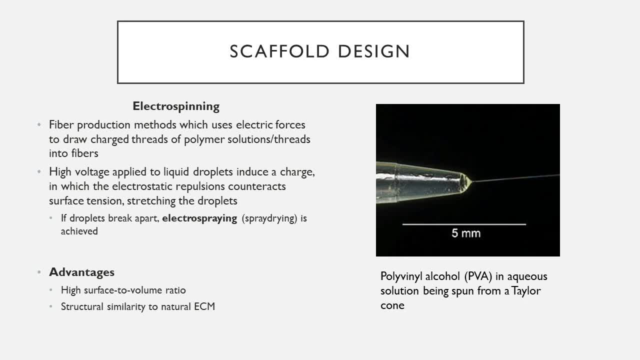 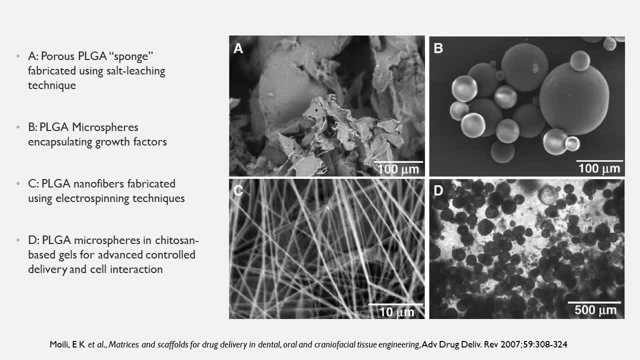 to the natural ECM fibers that you would find with natural collagen in typical ECM matrices. Now for this last slide. I've included a number of great SEM pictures of PLGA and PCL scaffolds and matrices and drug delivery vehicles. Excuse me So, in the top left picture. 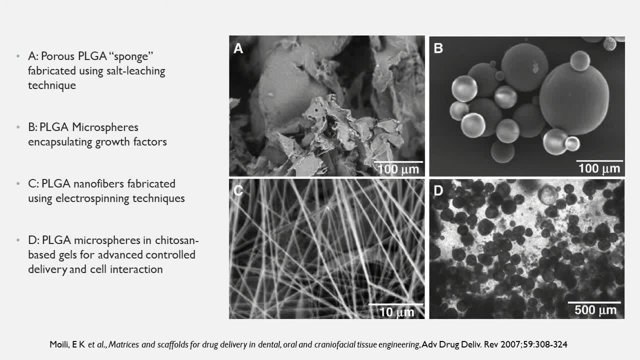 we have an example of a porous PLGA sponge which is fabricated using a technique known as salt leaching. Salt leaching are the use of salt derived porogens which would dissolve in the surrounding scaffold and then could be leached out just by submersion of that scaffold. 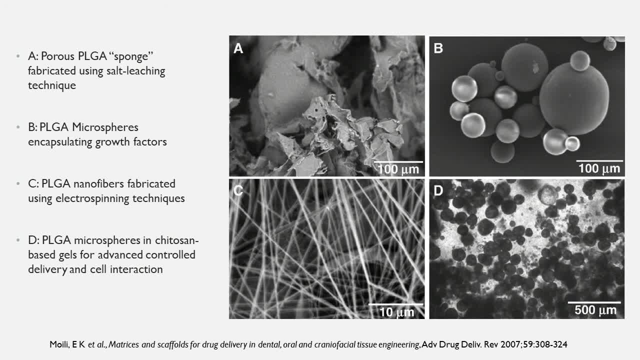 in water, So this would allow pores to be formed. then the salt would break down and then just leave the scaffold. In the top right hand corner we have an example of PLGA microspheres that can be made through a variety of different ways, in this case encapsulating. 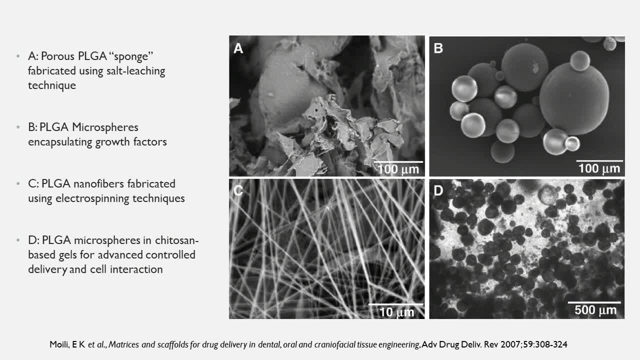 growth factors necessary for cells to regrow within the matrix. These PLGA microspheres are also very convenient porogens themselves, as PLGA can rapidly degrade depending on the amount of glycolic acid in it. In the bottom left hand corner we have examples of PLGA. 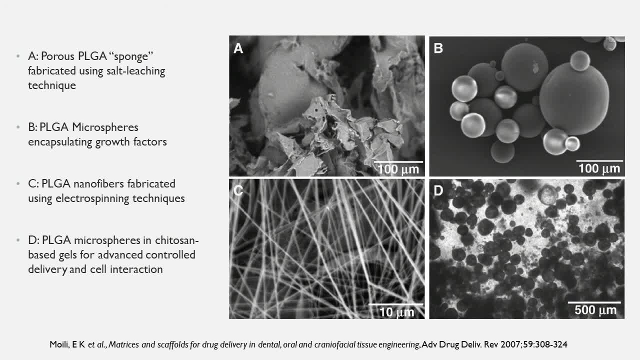 nanofibers that are made using electrospinning techniques, so you can kind of see their fibrous nature and how it might replicate typical collagen strands found in ECM matrices. And then in the bottom right hand corner we have PLGA microspheres that are 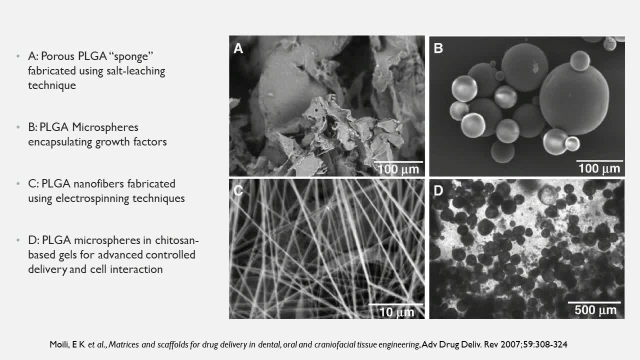 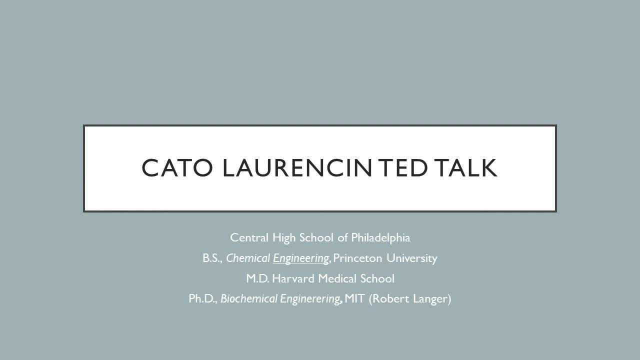 in chitosan based scaffolds for advanced control, delivery and cell interactions. Now for the last part of this lecture. I'm going to direct you to a different YouTube video of a talk by Professor Cato Lorentzen. Dr Cato Lorentzen, I should say. 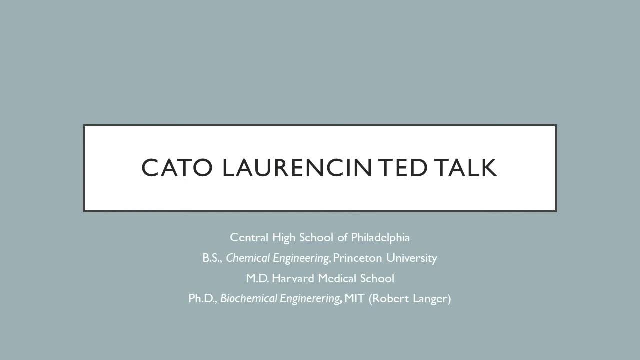 who's a product of our own Central High School in Philadelphia. He got his BS in Chemical Engineering at Princeton and then went on to Harvard Medical School and MIT for his MD and PhD. His PhD was from Bob Langer's lab at MIT. who's the subject? 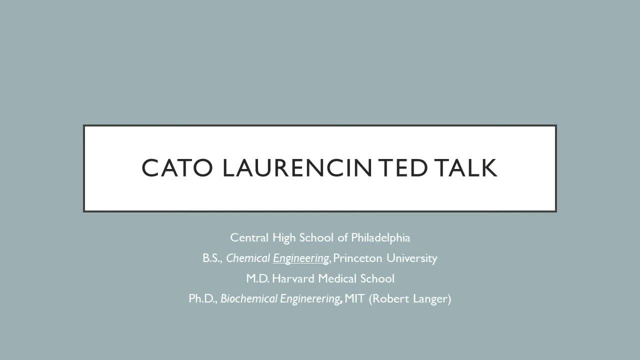 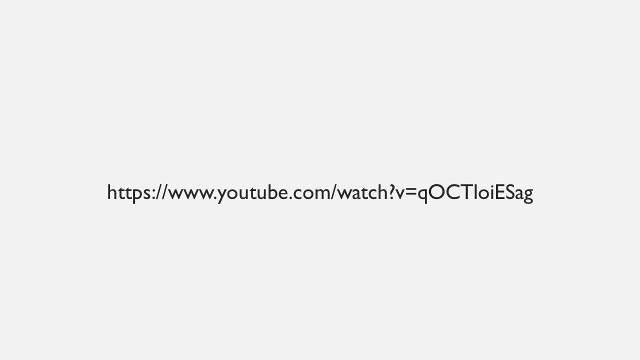 of the degradation YouTube video that Ted talked. So both of them are considered giants in the field of biomaterials in general: Cato Lorentzen. more on the biomaterials side, Bob Langer, both in biomaterials and drug delivery. But 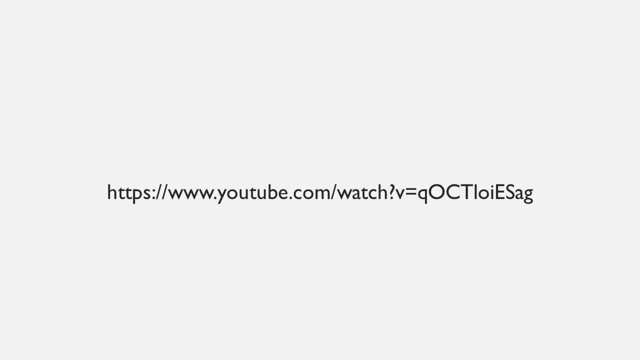 it's a very exciting talk, so I hope you enjoy it.